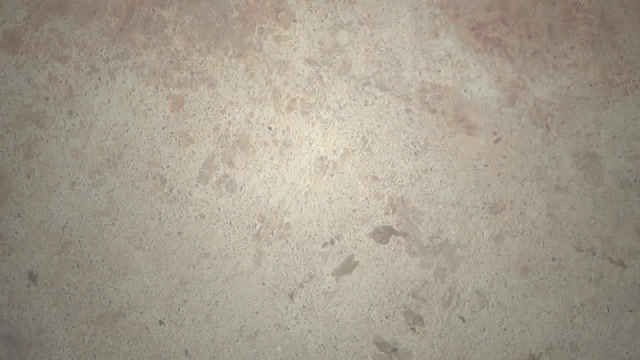 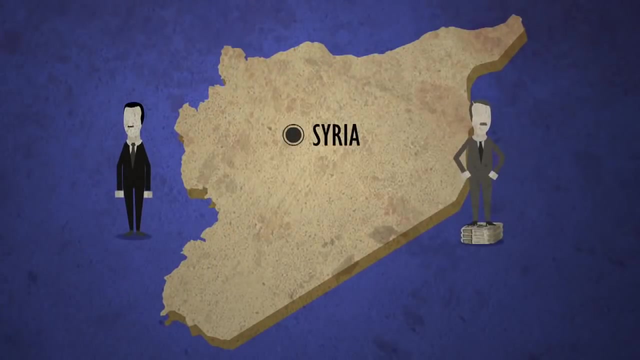 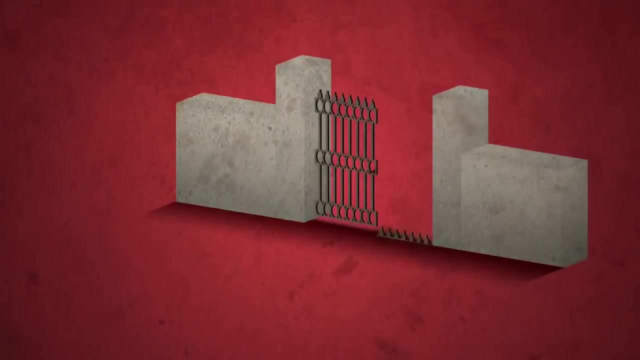 Muammar Gaddafi. Syria is another story. This is Bashar al-Assad, president of Syria. His father, Hafez, ruled for 30 years, during which he modernized the country, but at the cost of a brutal repression. Bashar came into power after his father's death in 2000, and at first he 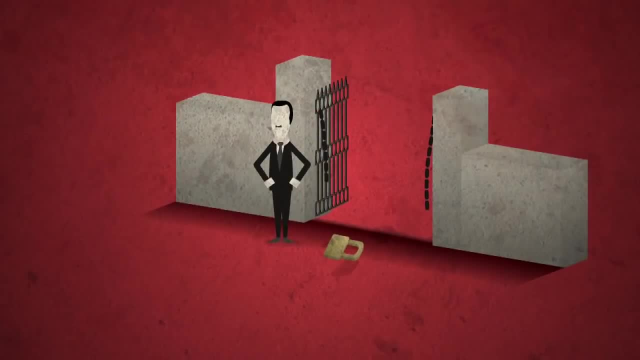 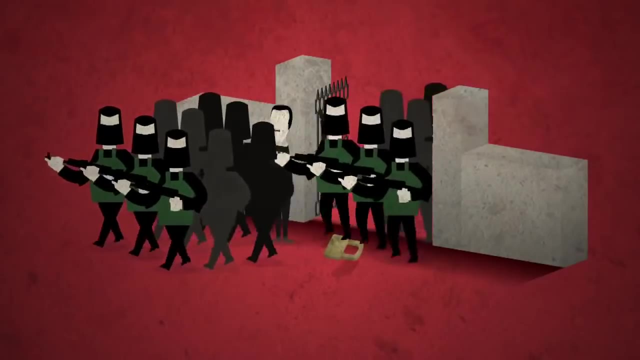 signaled he would be a different kind of leader, But the honeymoon with his people didn't last. At the first sign of dissent, Assad tightened the restrictions to free speech, isolated the economy and left very clear that democratic rule wasn't in his plans. 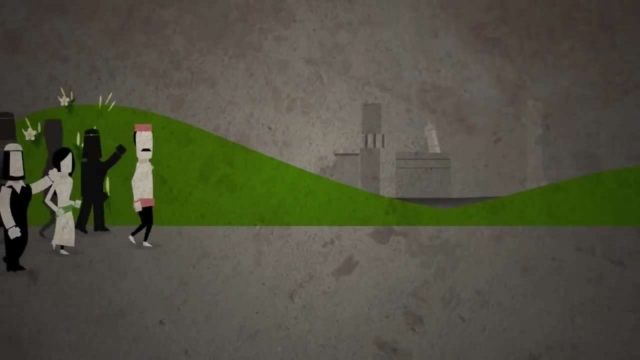 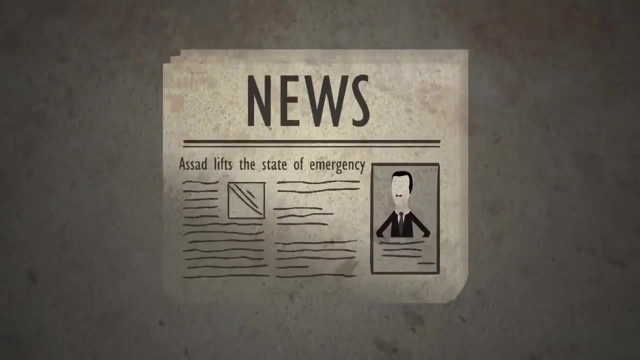 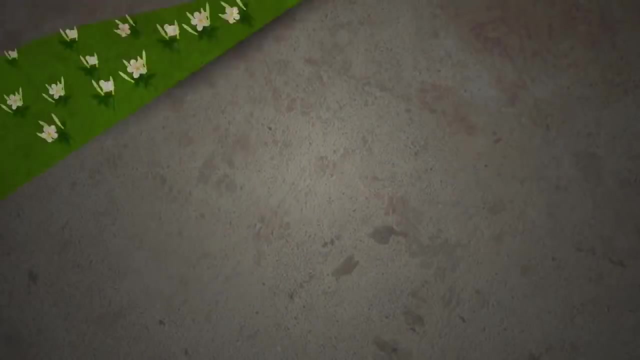 Twelve years of repression had to pass before thousands of people, following the example of Egyptians and Tunisians, took to the streets to demand reforms. At first, Assad's stance was conciliatory, but the repression continued, which in turn multiplied protests around. 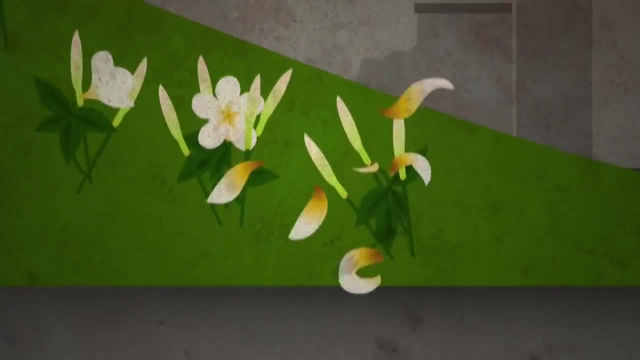 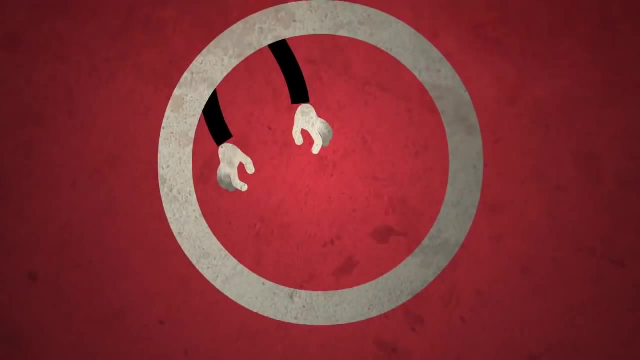 the country. The army answered by opening fire against the demonstrators. Hundreds died and thousands more were arrested. Any chance of a peaceful resolution died with the demonstrators. Small groups of armed rebels started to appear almost immediately. Since then, government and rebels are mired in a war of violence In Egypt and Tunisia. the uprisings led to. 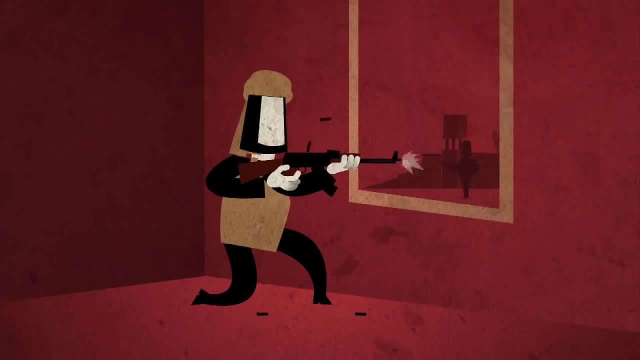 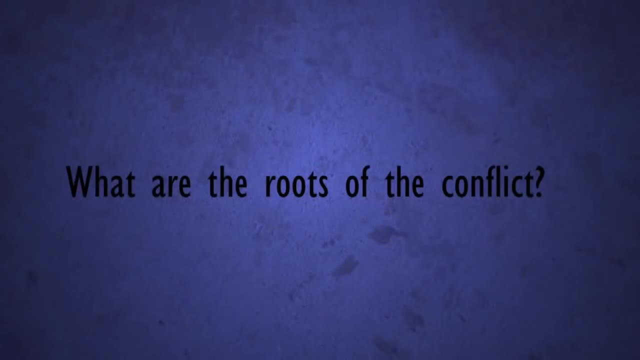 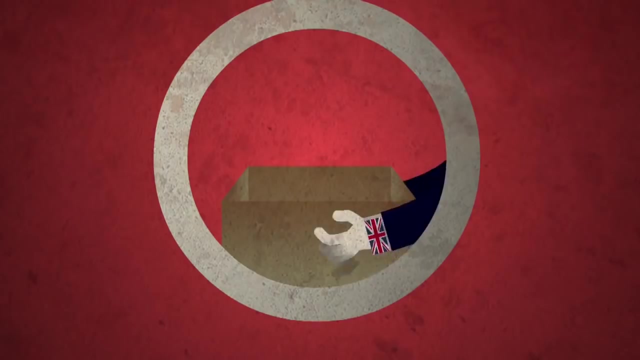 a war that claimed the lives of more than 60,000 Syrians. in the first 18 months of conflict After World War I, the French and the British established the borders of the Middle Eastern countries, grouping many religions and ethnic groups in the same territories. One of them, 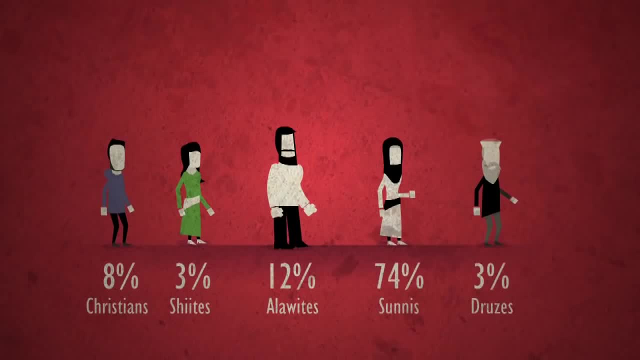 the Muslim sect of the Alawites has been in command of Syria since the 17th century. The Alawites have been the most powerful Muslim sect in the Middle East since the 17th century. One of them, the Muslim sect of the Alawites, has been in command of Syria since the 17th. 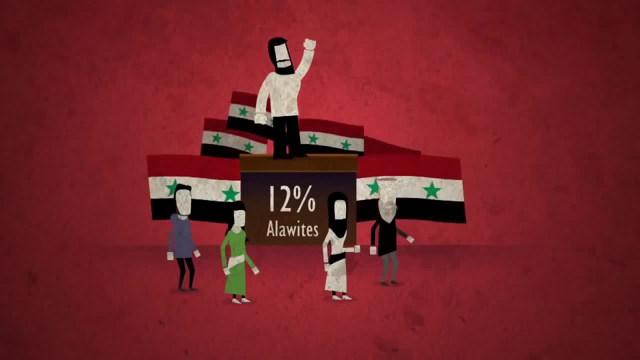 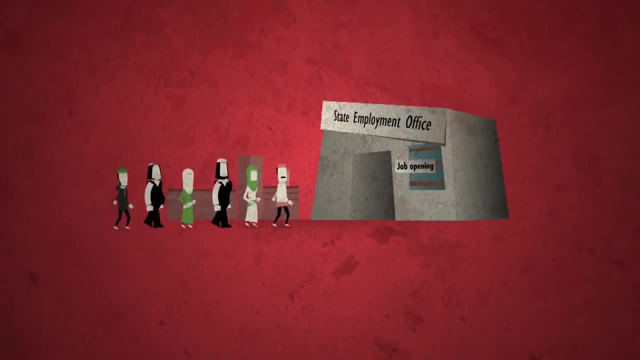 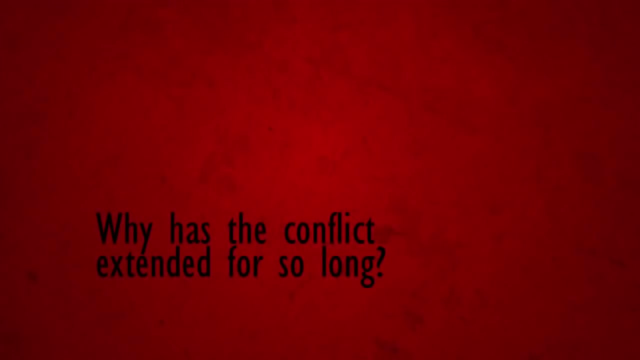 century. One of them, the Muslim sect of the Alawites, has been in command of Syria since the 17th century. The fundamental rule of the î naj-TF, which saved animals from being killed by its roots, isn subordinated to Islamism. 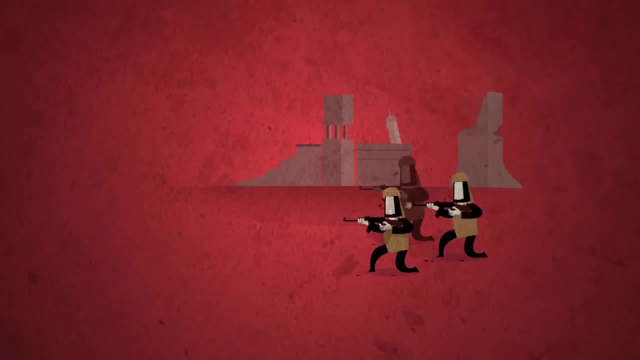 The deeply dominated Arab and Christian movements, carbs of absurdity under a changing strain of continual absolutism, The varieties of gathered anger and hatred across time, like the Sultanate of Jerusalem. But fight does not end with provocations. In 1990, terrorist attacks first emerged. 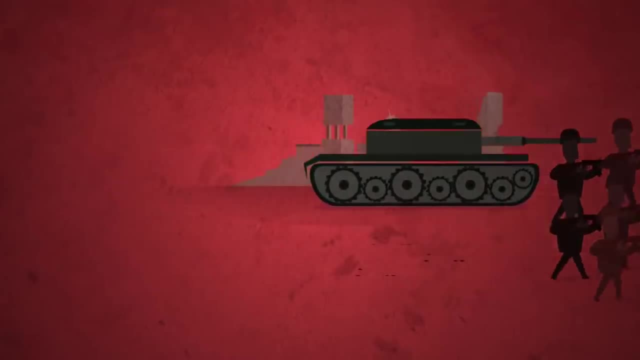 if you press Starroom, For the first time since 1977, groups have assembled by orden and group. This retkeiten is one of the most cricket-sized Islamic communities in gymnastics 밤 ideology. The only thing they have in common is a deep hate for Assad. 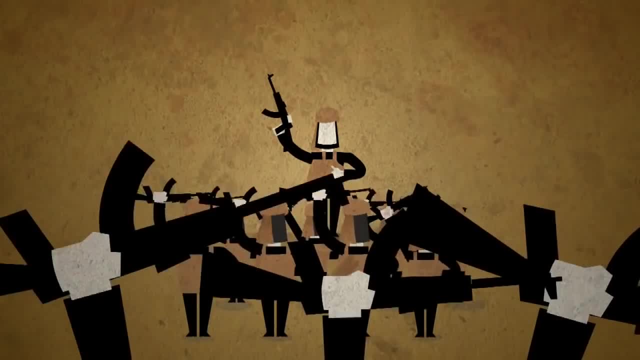 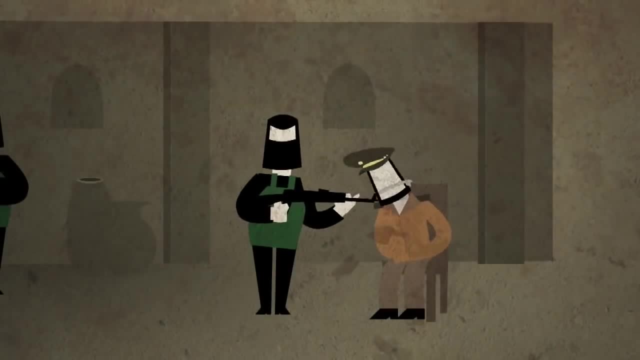 As the weeks and months pass, the rebels have increased in numbers and weapons, but not enough to topple Assad, who is now receiving help from Iran. Also, many of the rebel groups have abused, killed and displaced civilians in the name of the revolution, leaving many. 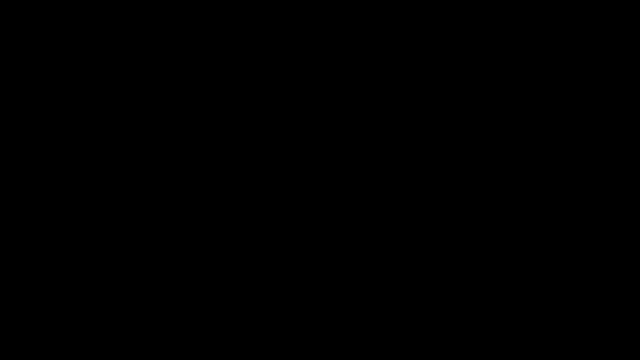 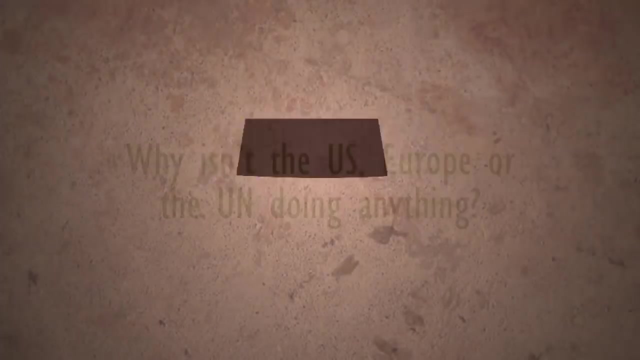 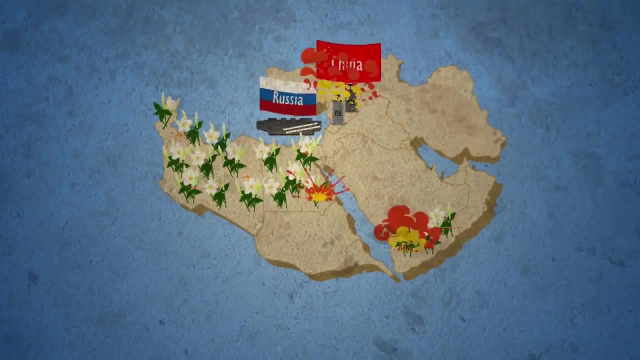 Syrians wondering if the cure is worse than the disease, Mainly because Russia and China have blocked any kind of international effort against Assad. Russia and China have interests in Syria and their leaders believe the Arab Spring hasn't brought security or stability to the region. The US hasn't intervened openly because it hasn't found a group who's aligned with its ideology and is wary that an intervention could give strength to radical groups. The experts believe that Assad will fall eventually. The question is how long it will take. 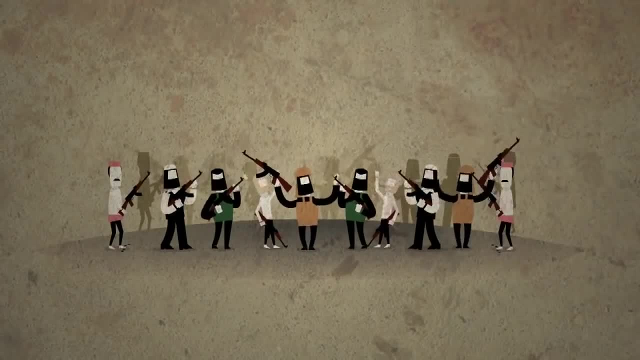 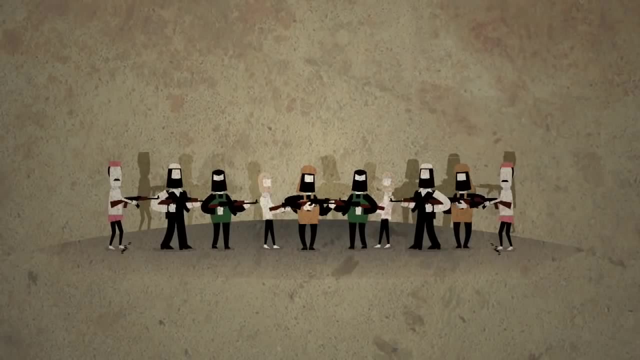 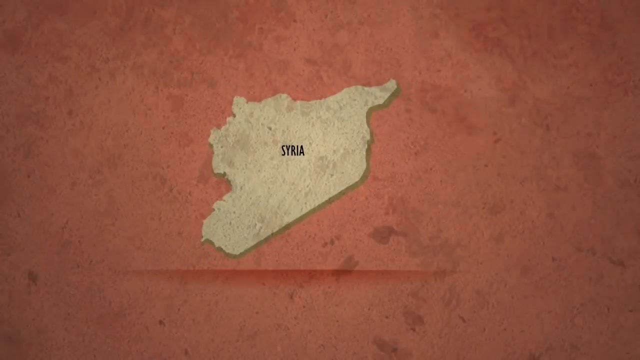 Although the main rebel groups have joined an alliance, it could crumble once Assad is ousted. The struggle for power could lead to a new civil war And even to a fragmentation of the country. The conflict could also extend to countries such as Turkey, Lebanon and Iraq, threatening 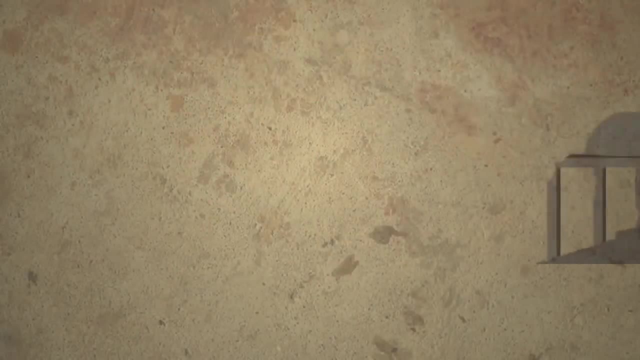 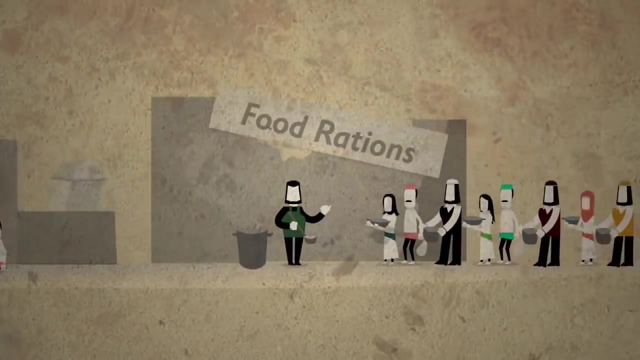 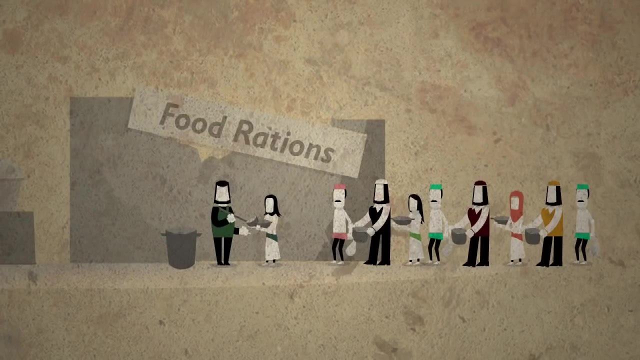 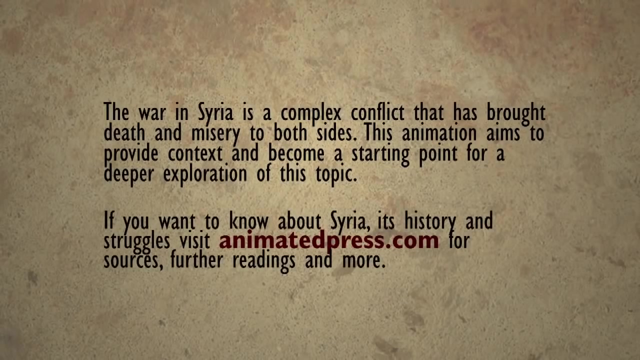 the fragile stability of the Middle East. No matter the outcome, whoever assumes power in Syria will inherit a country in ruins, with an economy in shambles, a deeply divided population and the challenge to fulfill the promises of the Arab Spring. It will be at this time that a nighttime war crumbles. 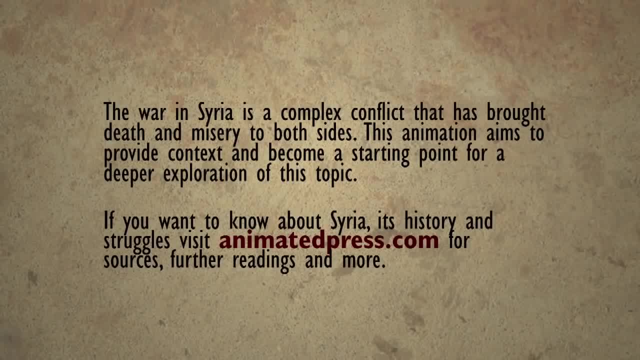 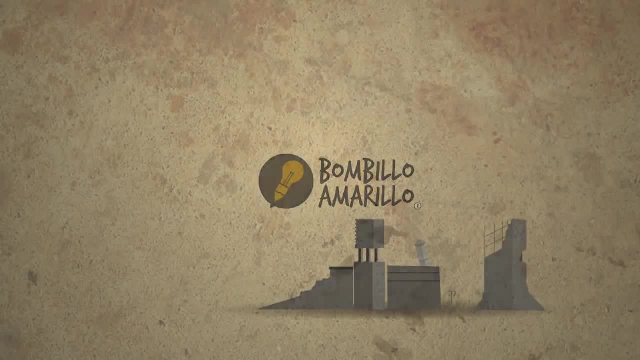 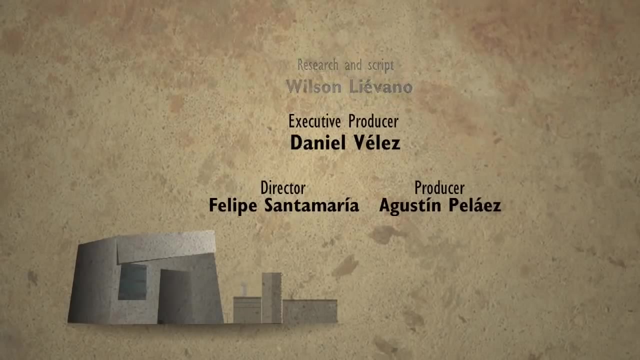 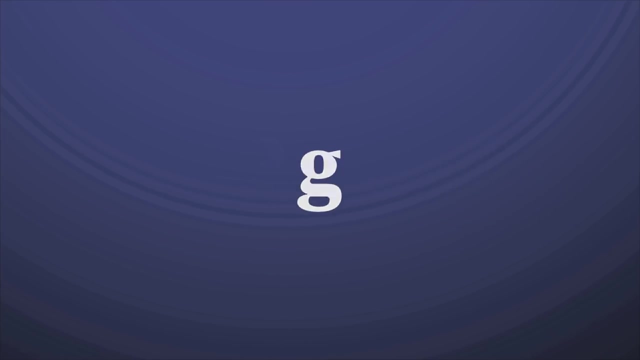 In April, letzte Mature will torch the passive lives of millions of hungry children as they starve to death in the eastward of Afghanistan. jogo Story: Se règimen изб concret Lq Wild Ok, prestigious, It's time not to scare. We'll be right back.